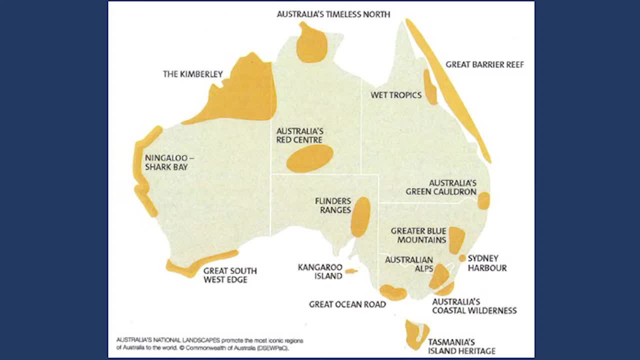 national landscapes. Now that was a concept to promote tourism and heritage and visitation and national parks by the federal government about a decade ago. We have the Flinders and Kangaroo Island in a big space in the middle And I'm not very impressed with the space, but it's a lot of space. 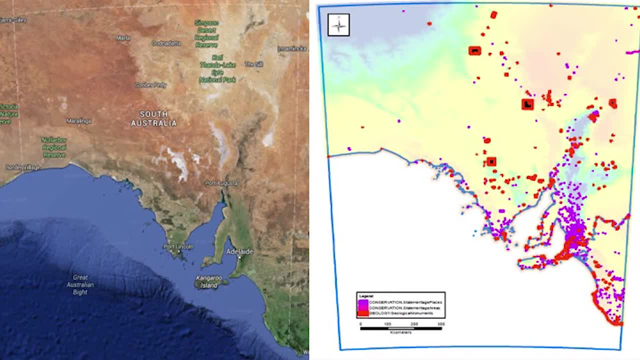 If you look at the map of South Australia here, you all know where Kangaroo Island is because it's labelled, and you can follow the curve of the spine or the backbone of South Australia, up through Adelaide, up past Port Augusta, right up to the top of the Arca. 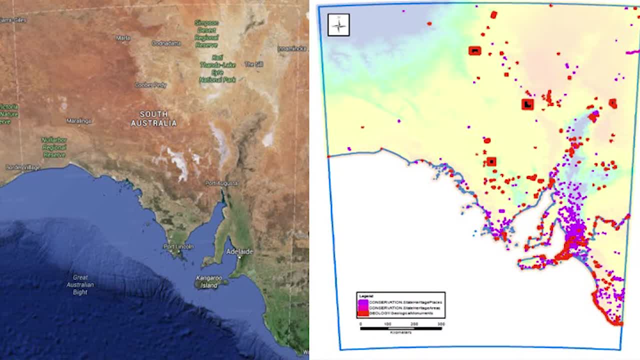 Rula, where the Flinders Ranges are, and all the coloured dots are geological sites, heritage sites, places of importance in South Australia. There's so many of them that would fit into a trail. I haven't got a bat big enough. 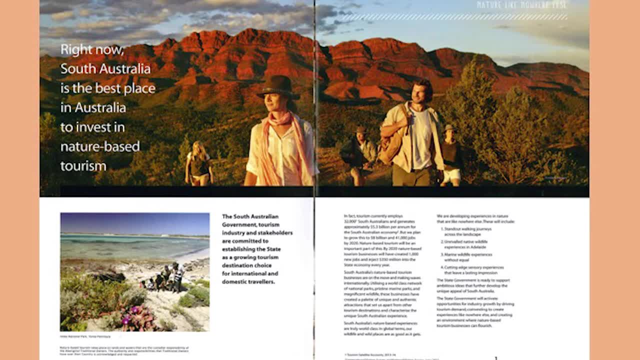 Pinched this out of one of the Virgin magazines just promoting that South Australia is a damn good place to come and have a look at, and the backdrop is this whacking great red sandstone range. I'm inspired by that. I hope you are too. 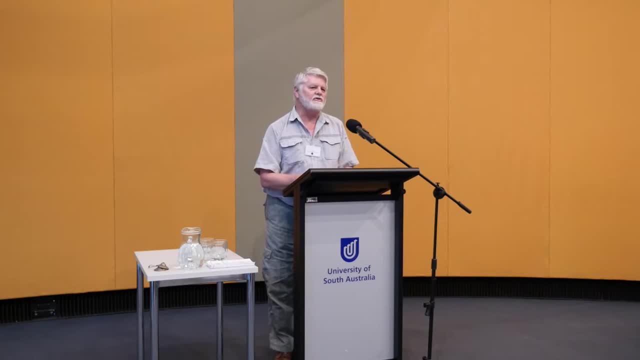 I'm going to take you on a very quick trip along the spine of South Australia, which I call a song line, if you like. an S-shaped backbone of South Australia Starts at Remarkable Rocks, and those rocks were rocks that saw Gondwana and Antarctica. 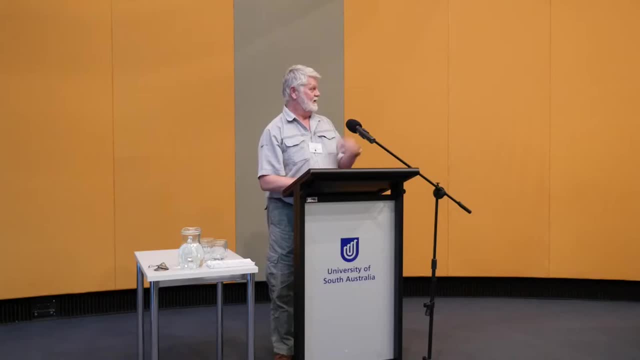 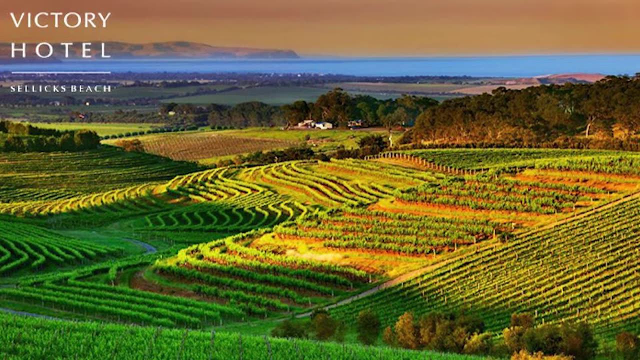 before we broke, And that is the beginning of that story. We're standing here at the Victory Hotel, which is one of the best pubs in South Australia, because it has an absolutely beautiful view, but it's on the Willunga Fault Line, so 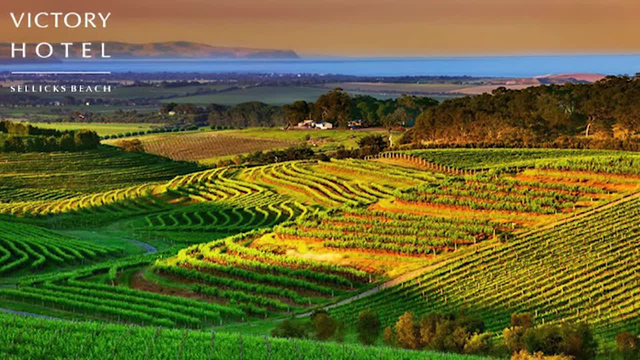 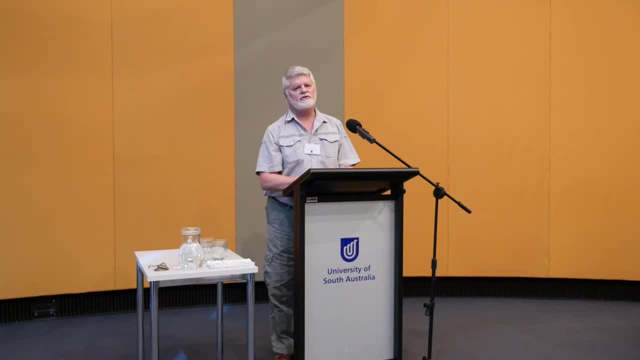 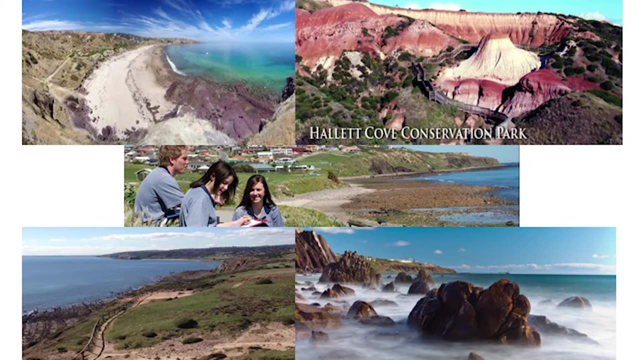 for geologists. we think that's fantastic. But you can look across all the soils that are generated by the fault blocks of the Adelaide Geosync Line, which have generated all those beautiful vineyards and so on in the McLaren Vale area. Tiny Little Hallock Cove is a really high profile, very important geological site which 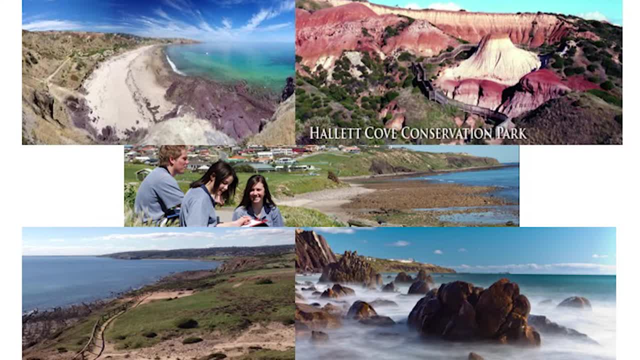 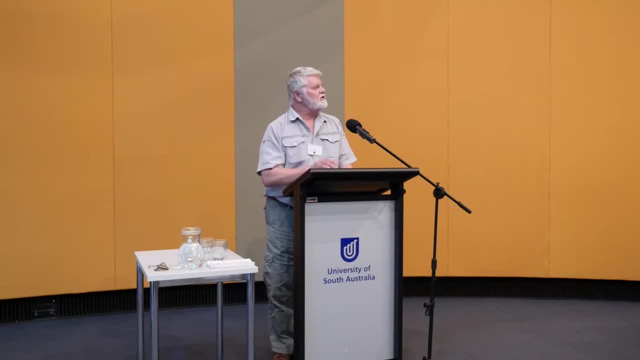 covers from 500 million years ago up to the present, But it's got a city of a million people around it, so it is a prime location for being supported as a place of excellence and a UNESCO Geopark which can be supported by communities of that. 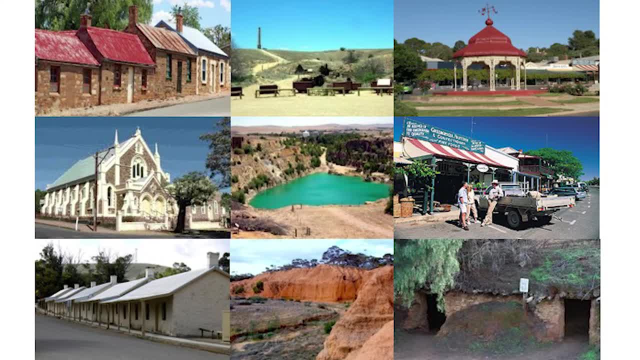 order, Zooming up the middle of the state because we're on a rush trip here. here are a range of images from Borough- and the Minister mentioned this morning about the Borough Charter, commencing here. A whole range of different experiences, Whether they are geological and regional. they are geological and regional. they are. 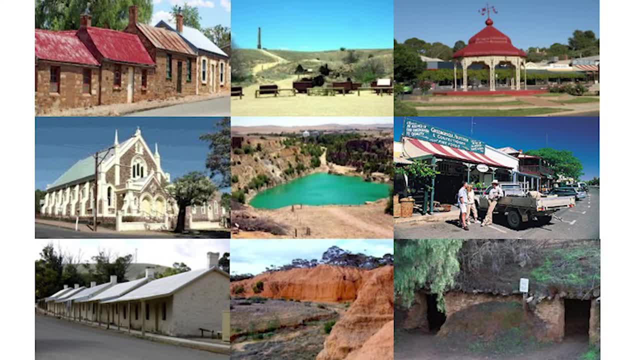 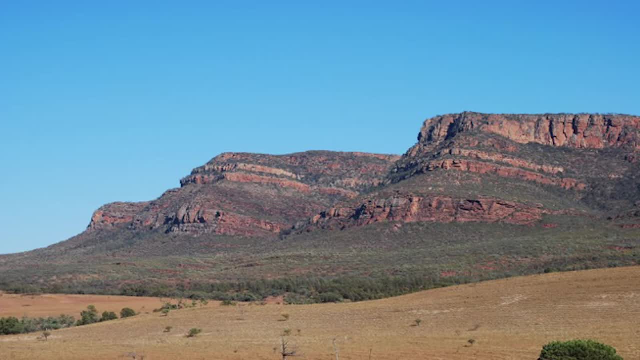 geological and regional, Whether they are in relation to the mines or whether they are historical. I'm racing up the Flinders Ranges to Rawnsley's Bluff on the edge of Wilpena Pound. The caption on the photograph said that was Dutchman's Dern, but it's not. 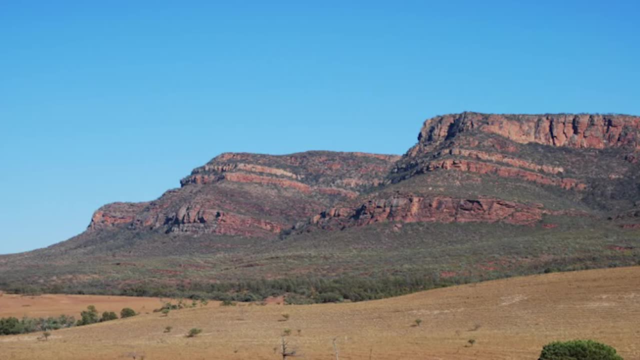 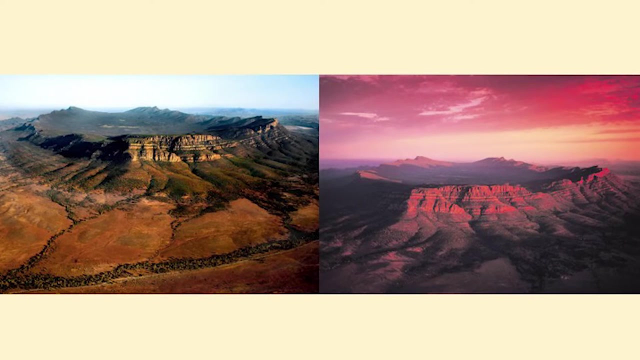 These are dramatic ancient landscapes and that is part of our story. The geological story is effectively history before the history. The human history is a small bit at the end. Wilpena Pound, we all know and love. There it is in the morning and later in the day. 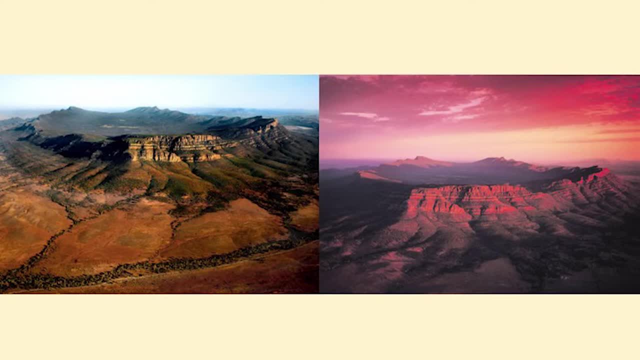 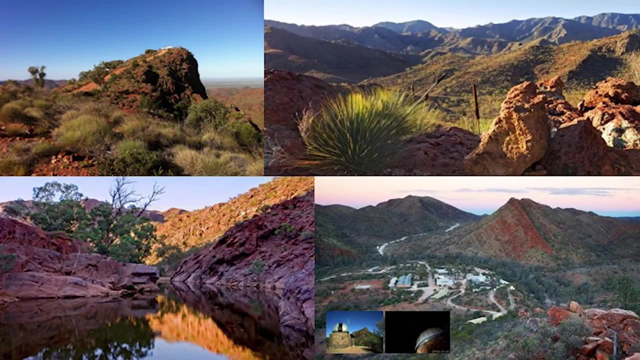 It's just too good a slide to lead off, basically, but we're talking about long distances. to try and promote visitation, We need to look at concepts such as aerial tours that become much more available to appreciate our landscape, That composite there is of Arcaroola at the top of the Flinders Ranges. 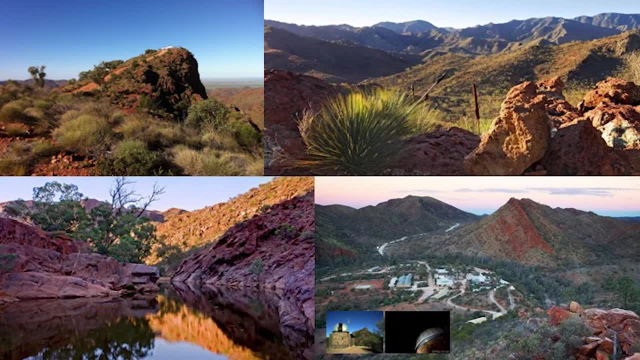 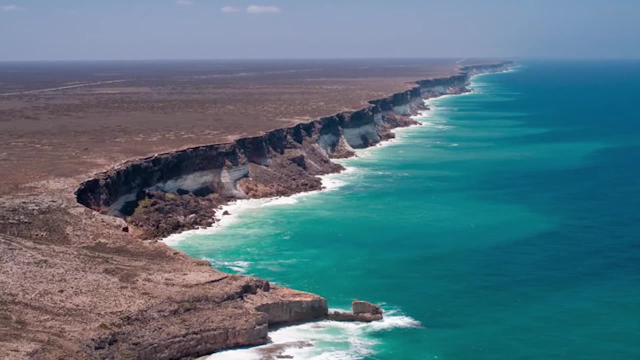 Just different sites and different experiences that visitors can have when they stay at Arcaroola and those tiny little stamps down the bottom are, at night time, looking through the observatory at the southern skies of Australia, which is just a brilliant experience. This is an alternative concept to a trail running up the middle of South Australia. 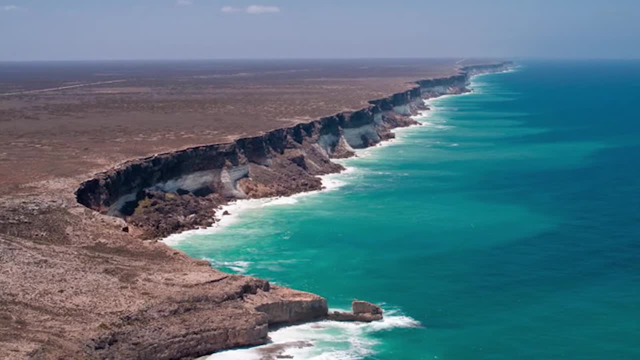 It's looking along the coast from west to east, The giant cliffs of the Nullarbor and the whales, of course, that come there. Why do we have cliffs there? Because Australia, at our end, is lifting up and digging down at the front, past New Guinea. 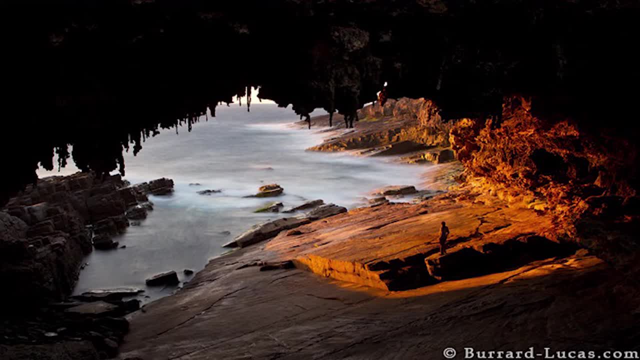 So that's why we've got the cliffs, Kangaroo Island, we have the cliffs, And here we have the Nullarbor, The Admiral's Arch with those stalactites, which is a very new, young piece of rock which geologically happened last week, resting on that pavement where he's standing, which broke. 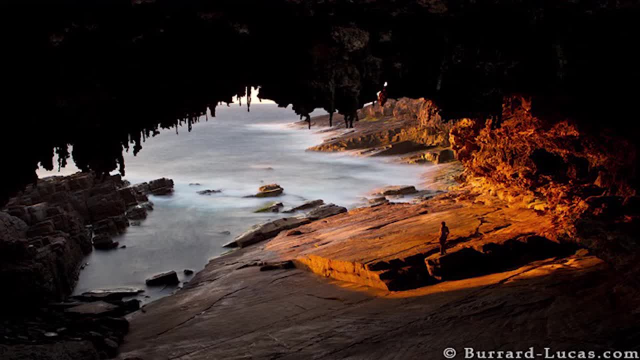 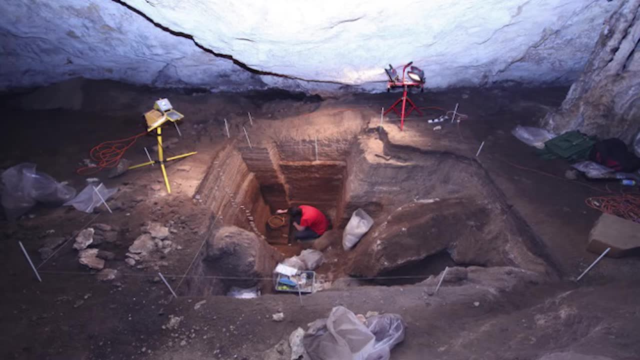 away from Antarctica 60 million years ago And if we zoom down the coastline towards Narragor, there's my friend Dr Liz Reid in the bottom of a pit. You see the little white tags there. She's looking at different layers in the sediment that go back half a million years and we 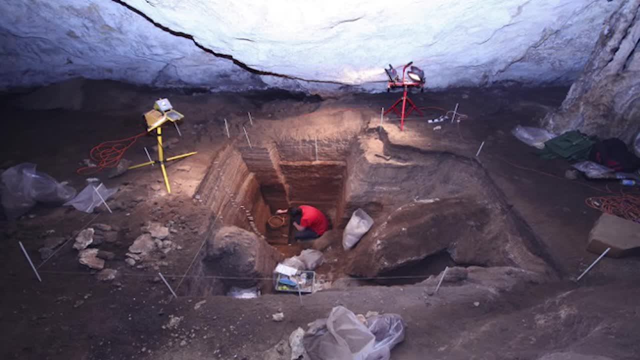 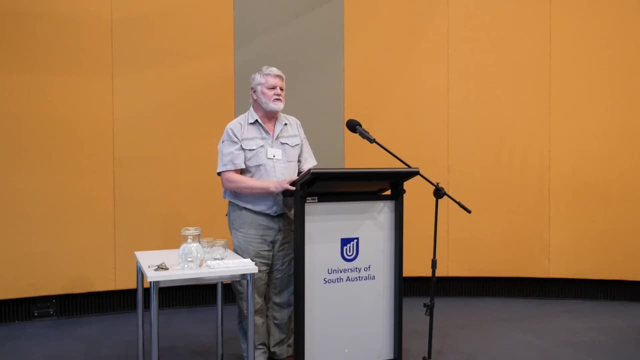 are looking now at experiences, Experiences where people can pay to sit alongside the paleontologist and work with them, even if it costs a lot, and they work with the professional and they share in the discoveries. Narragor- I've put this in simply because it illustrates some of the fossils for which